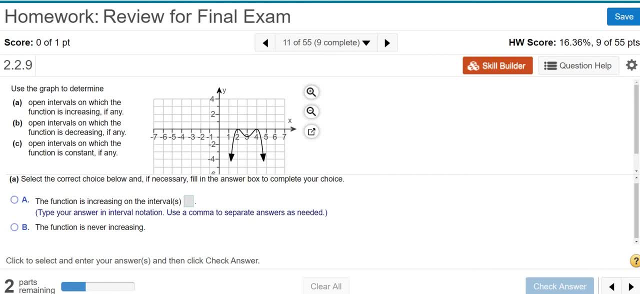 It says: use the graph to determine. So part A, open intervals on which the function is increasing, if any. And then here it wants us to fill in the answers. So increasing, let me make it big so you can see it. So it's getting bigger here and it's getting bigger. 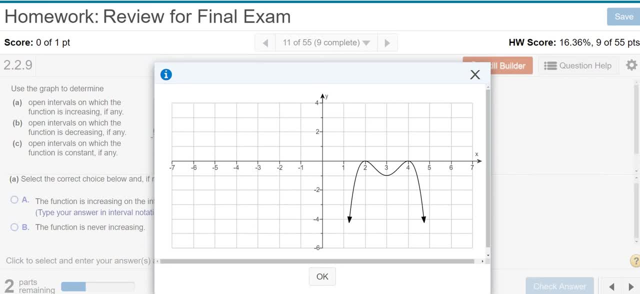 here These two little pieces, If you look at it, left to right, big, big, big, big, big, big, big, increasing, decreasing, increasing, decreasing. So from negative infinity to 2 it's increasing. and also from 3 to 4 it's increasing. So negative infinity to 2, increasing. 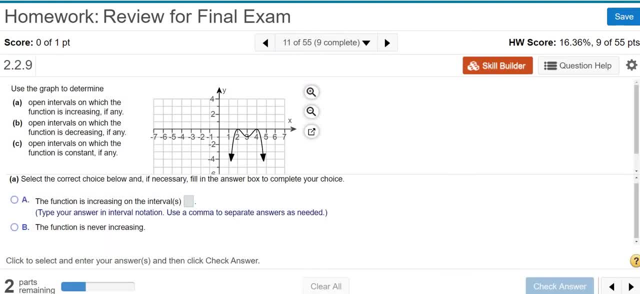 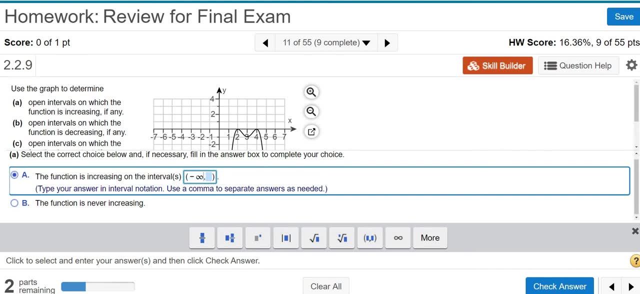 3 to 4, increasing. So I'm going to go ahead and type that in here to make sure it's correct. So parentheses and then negative infinity to 2. we said- And you can still see it here, Right, You can still see it here in the picture, And I'm going to put a comma. It says use: 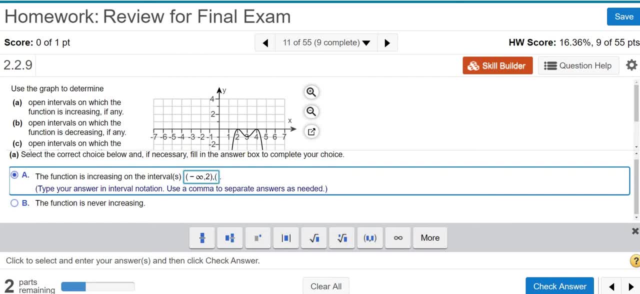 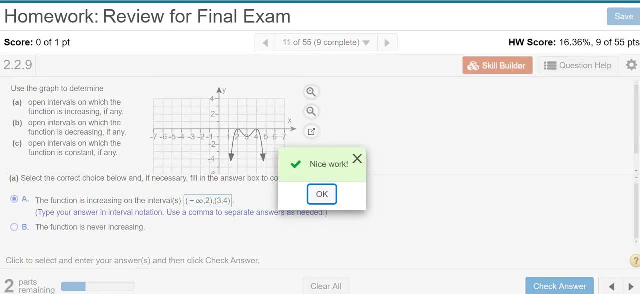 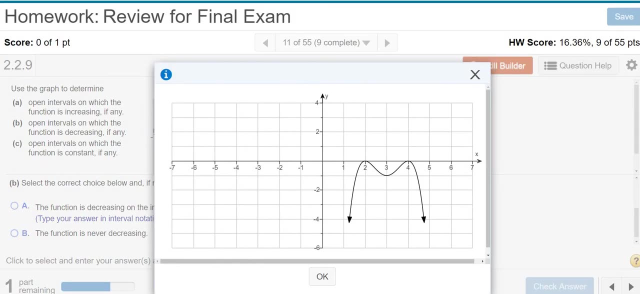 commas to separate answers, Good, And then 3 to 4 and then parentheses, And let's click check answer and cross our fingers: Boom, Nice work. That's how pros do it. Now we want to know where it's decreasing, So let me make it big so you can see it. So right here you. 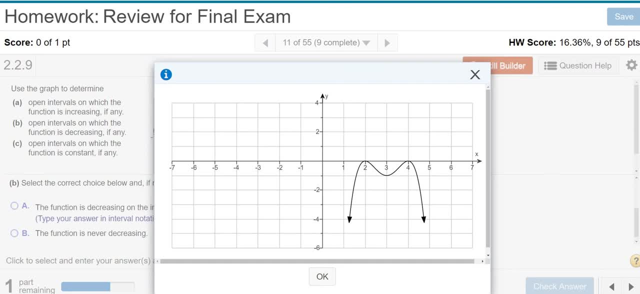 see it's getting smaller from 2 to 3.. It's always x values, So from 2 to 3, the y values are getting smaller. From 4 to infinity, the y values are getting smaller. So 2 to 3 and 4 to infinity, Notice. 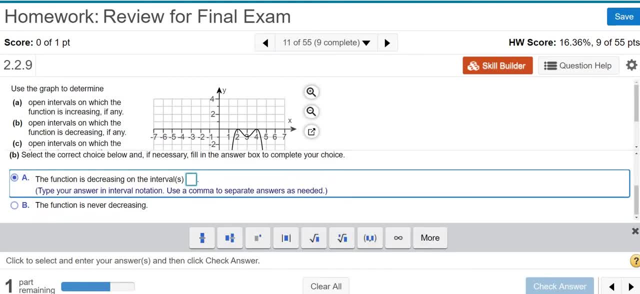 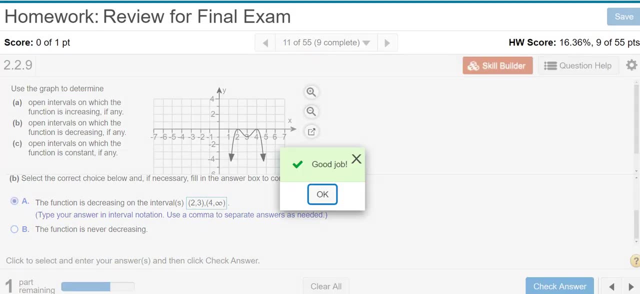 that I'm using parentheses for the increasing decreasing. It's super important to always use parentheses for increasing decreasing, Always, no matter what. Let me just double check: 2 to 3 decreasing, 4 to infinity decreasing And moment of truth, Boom. Good job Select. 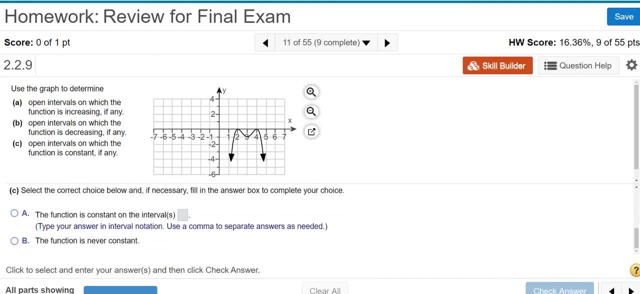 the correct choice. Next one is constant. Constant would mean it's just like a horizontal line. It's not changing, So it's never constant. So I'm going to click this one Check answer And that's it Next question. Good job, I hope this video has been helpful.